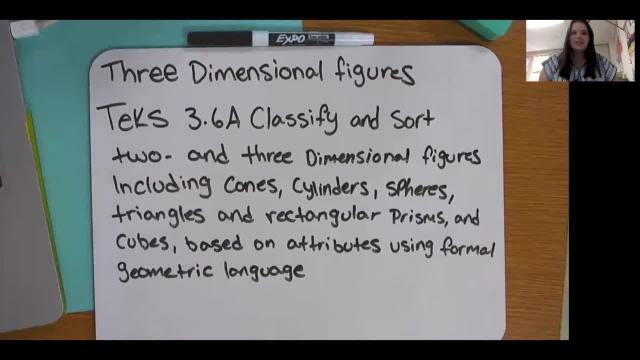 Hey guys, it's Ms Lopez, and during our last lesson we learned about two and three dimensional figures. We learned what they were, we learned how to identify them, and today we are going to learn how to identify the faces, the edges, the vertices and the bases of three dimensional 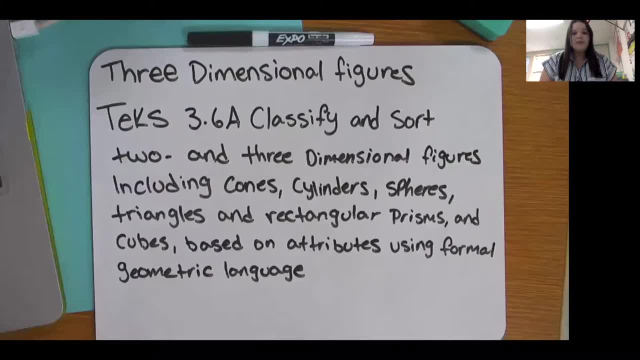 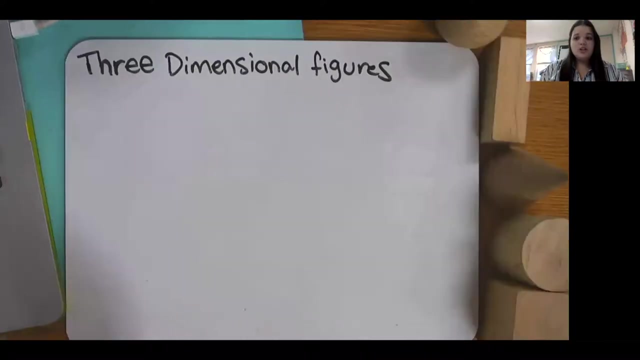 figures. So the teak that we're going to be using today is teak 3.6a. It reads: classify and sort two and three dimensional figures, including cones, cylinders, spheres, triangles and rectangular prisms and cubes, based on attributes, using formal geometric language. So we are going to be learning. 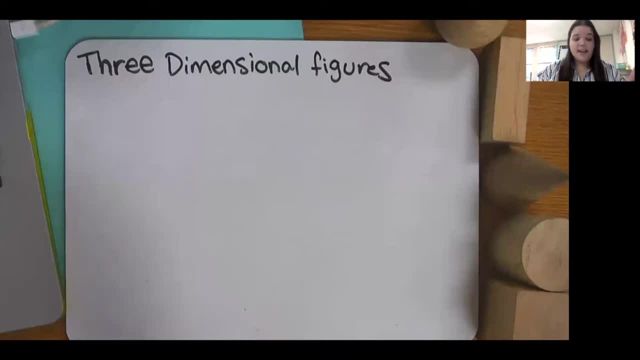 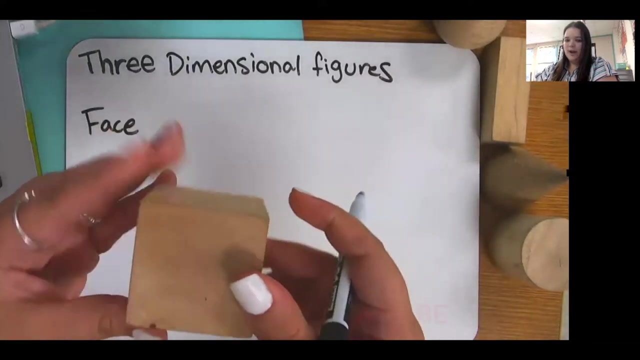 how to identify the face, the edge, the vertex and the base of a figure. Now, the face is any flat surface on a solid figure. So let's say I have some examples here. Let's say you have this right here, This is a square. 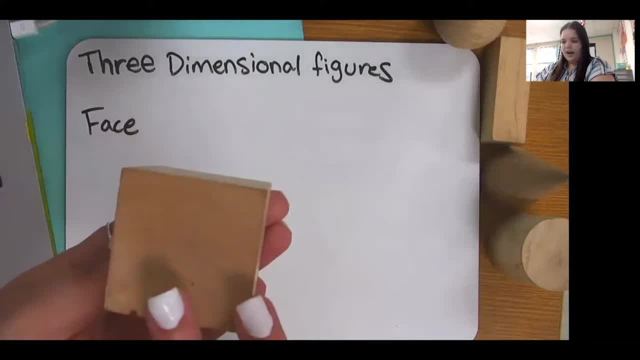 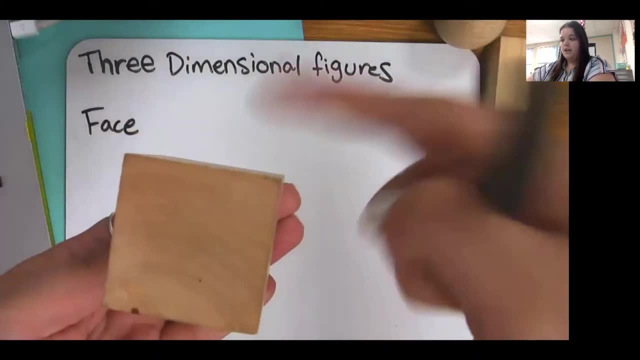 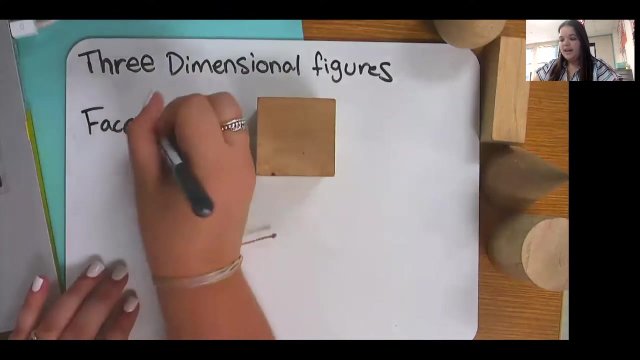 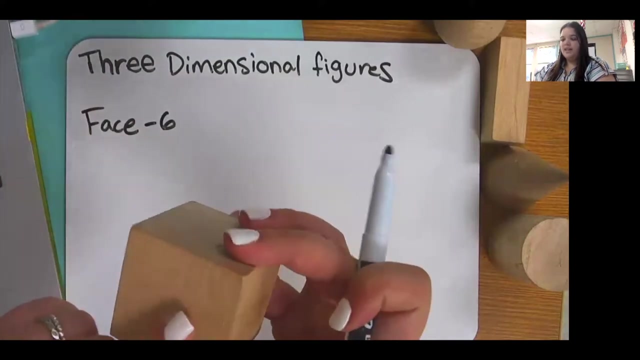 So you're going to count how many faces this square has. So you're going to go one, two, three, four, five and six, the bottom one. So how many faces does it have? The square has six faces. It's any flat surface, any flat surface that the solid has, that the figure has. 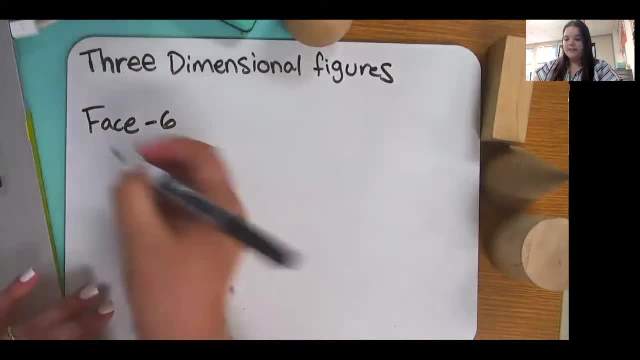 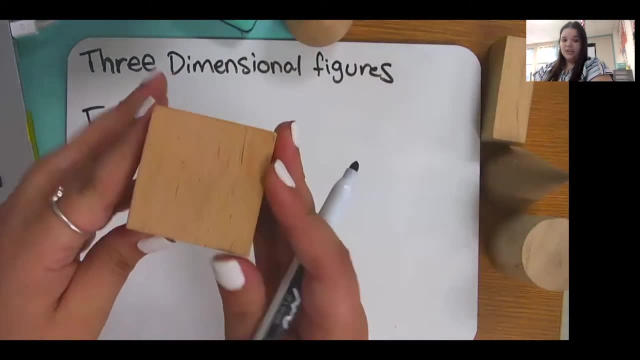 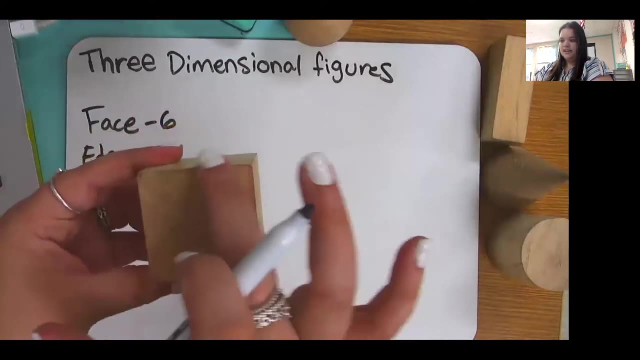 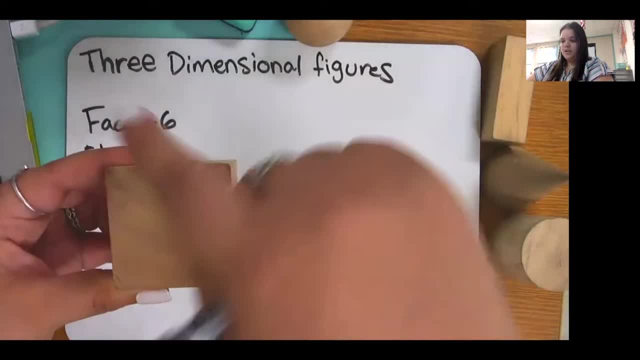 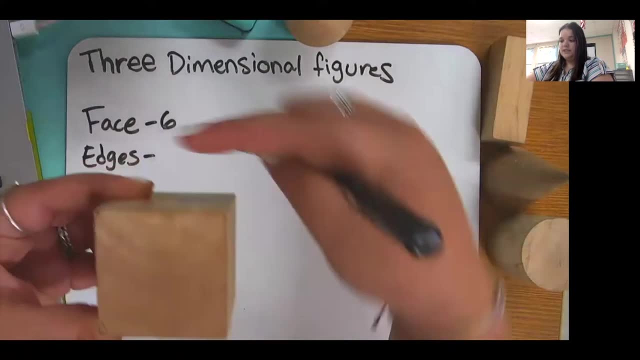 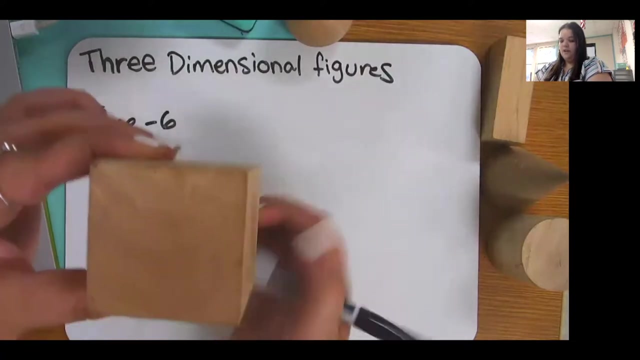 those are what you're going to count. So you're going to go one, two, three, four. You're going to go sideways five, six, seven, Eight and then, at the bottom, nine, 10,, 11,, 12.. So how many edges you got? You got 12 edges. 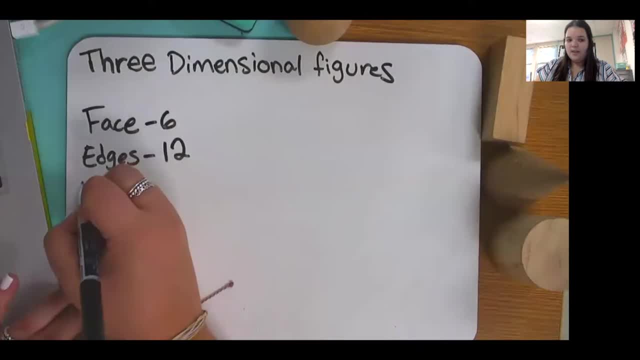 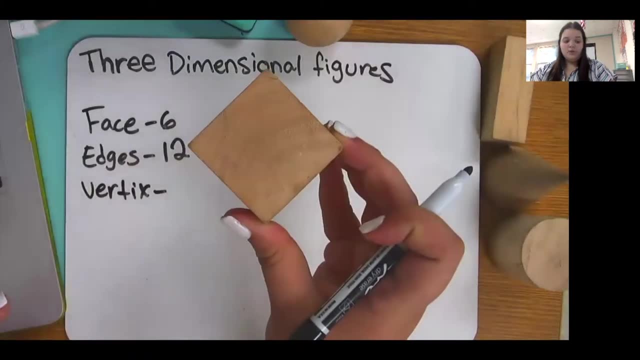 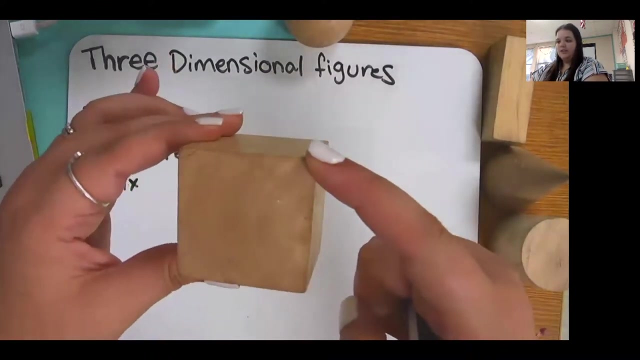 Now, once we finish with the edge, now we're going to go with the vertex. Now, the vertex is the corner in which three or more edges meet. The corners would be this one, right here, You see, it has three edges meet: One, two, three, four, five, six, seven, eight, nine, 10,, 11,, 12.. 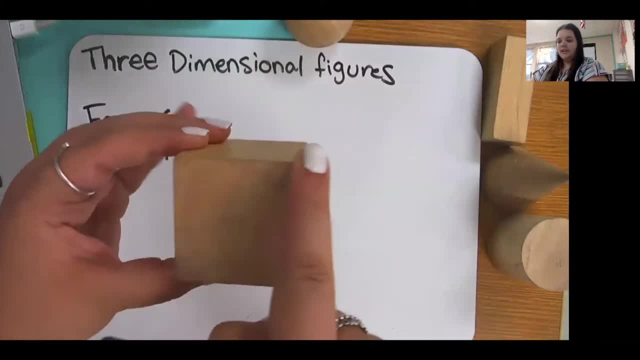 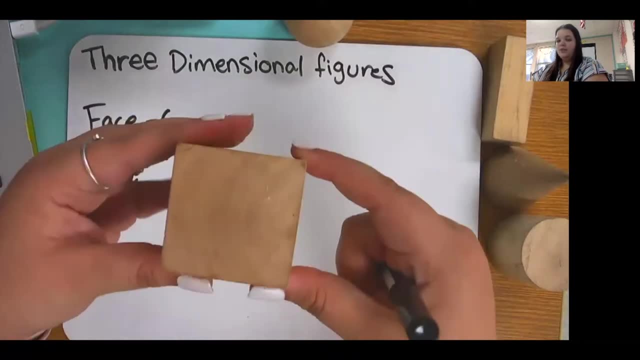 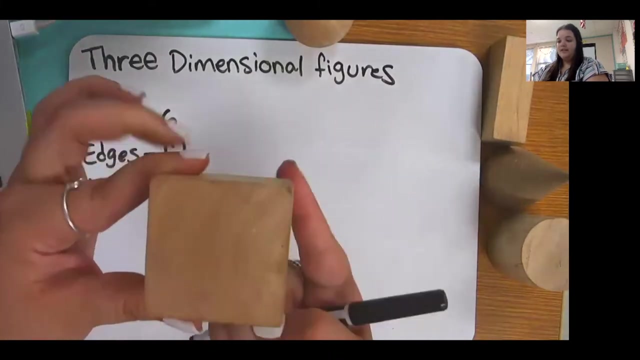 So that is one vertex, This is another one. One, two, three edges meet, So we're going to count the vertices One, two, three, four, five, six, seven and eight. You got to count the bottom. 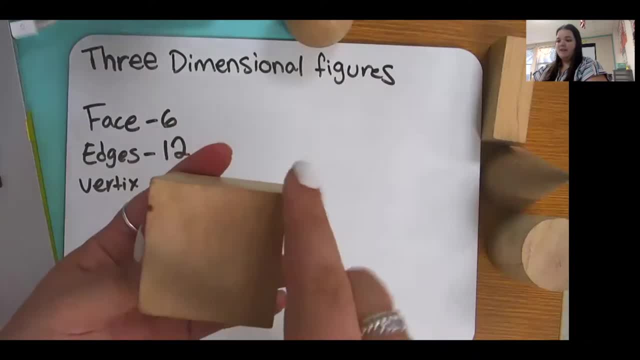 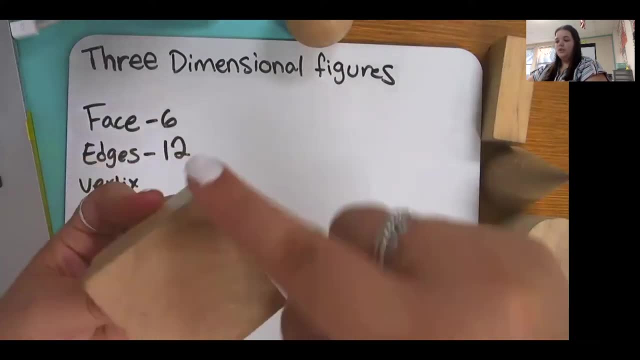 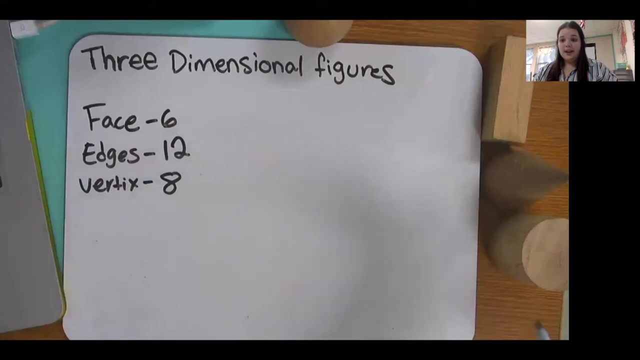 ones too. So if you flip it, you're going to have the same amount of edges. So one, two, three, four. one, two, three, four, So you got eight vertices. So now we know that a square has six faces, 12 edges and eight vertices. Now let's see. let's try with another figure. 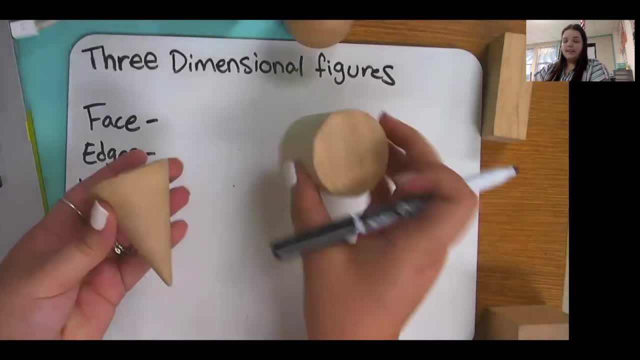 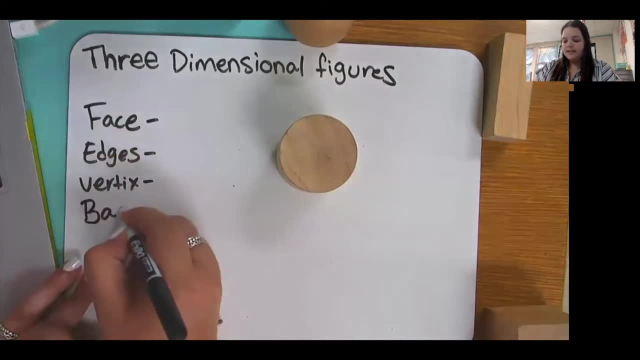 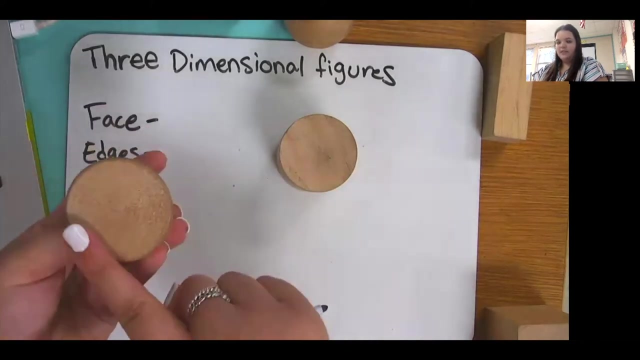 Now the cone and the cylinder. they have a different one, They have an additional one that is called a base. So the base of a solid figure is a flat surface. So how many flat surfaces does a cone have? So it has one. this is all flat, and two. 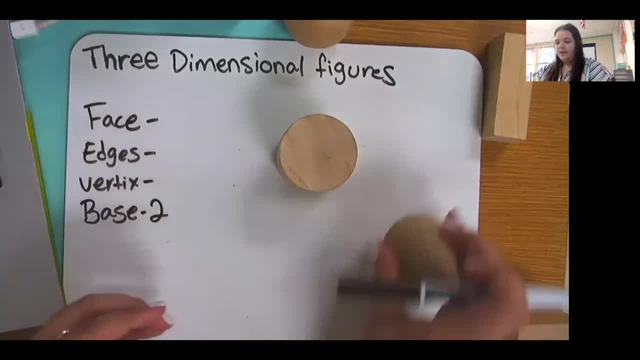 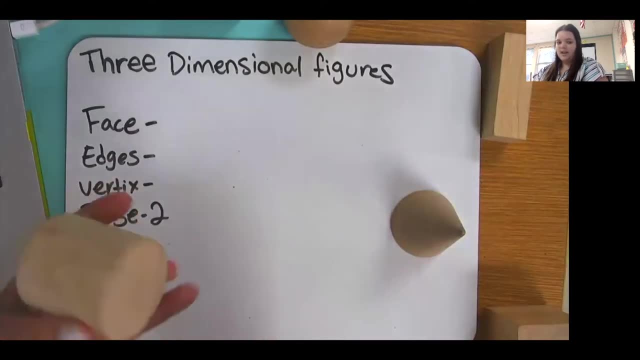 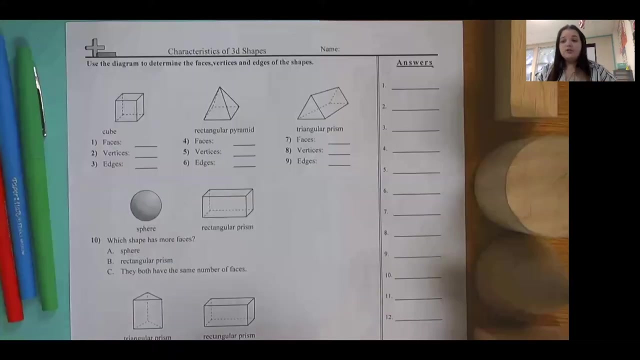 So it has two flat surfaces. Now, how many flat surfaces does a cylinder have? It has one, two and three. So that's how you tell the base of a solid figure. Now, using this worksheet that I have already handed out to you guys, we are going to count the faces. 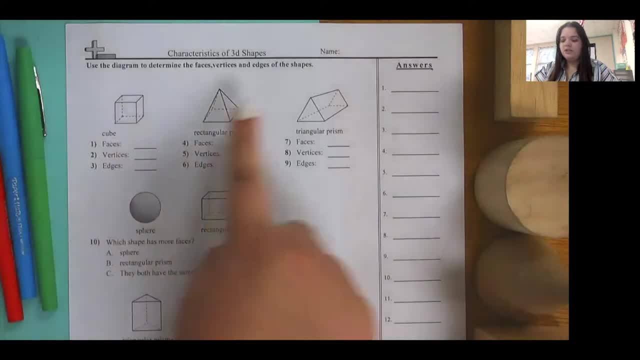 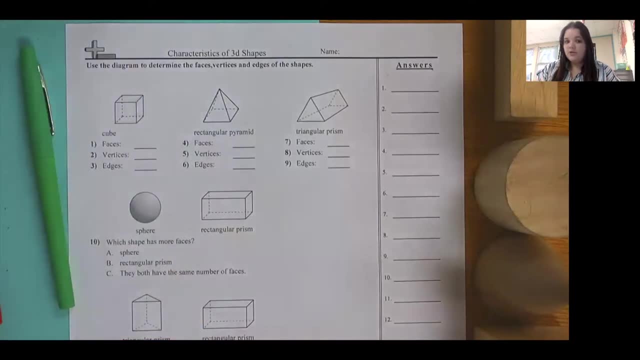 the vertices and the edges of those particular shapes. Now we have. how many faces does the cube have? So which ones did we say were the faces? This is flat and two arm and legs. So now we got eight faces. 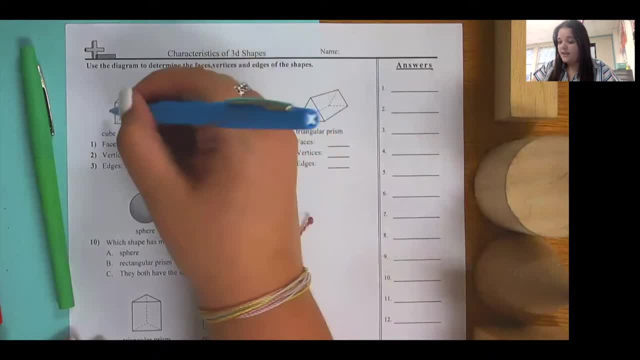 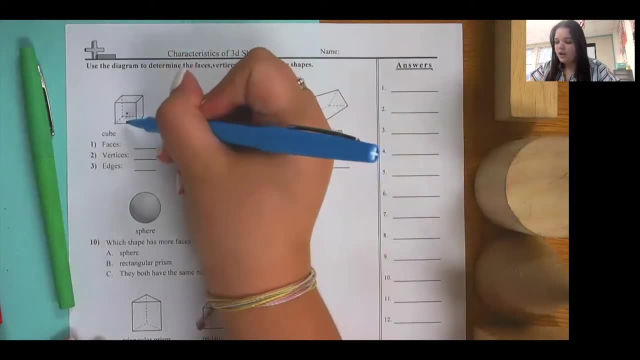 face, this is a face, the one behind it's a face, the other one is a face, and this is a face. So we're going to count those faces right. So we got one, two, three, four, five and six. So we got. 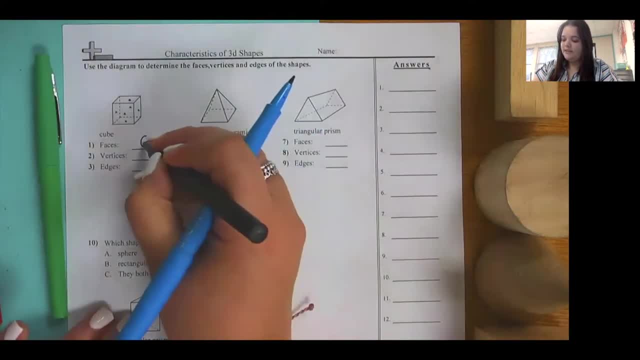 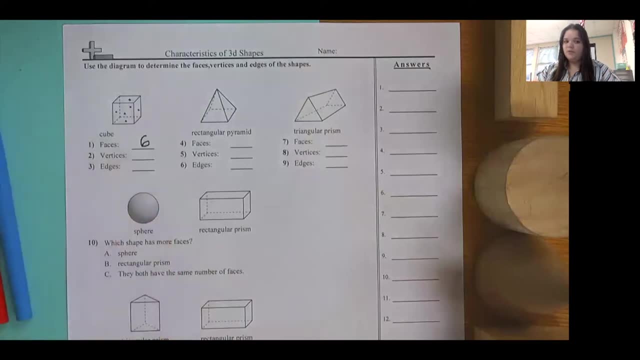 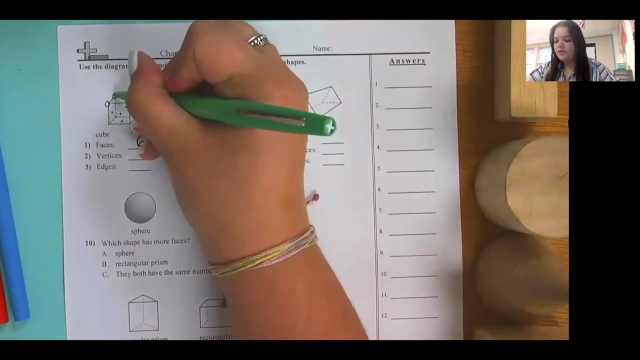 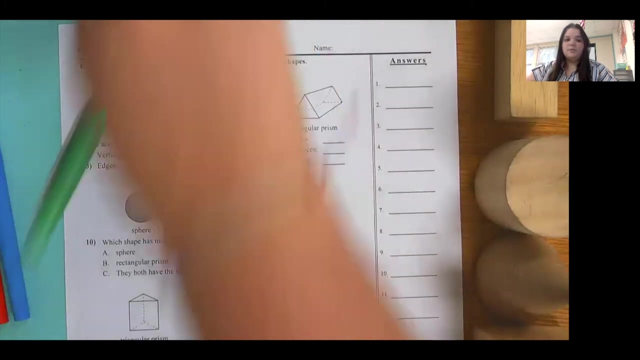 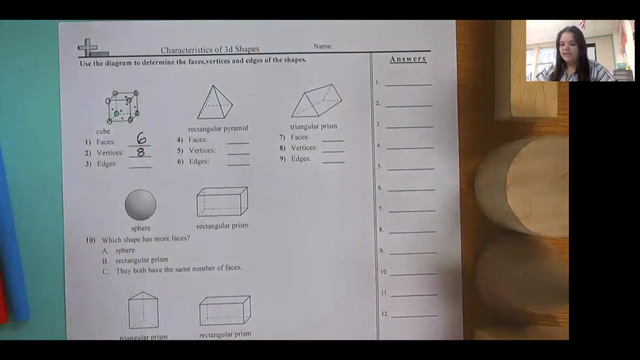 six faces. Now, how many vertices do we have? Which one did I say? were the vertices, The corners? Good job, So the corners are one, two, three, four, five, six, seven, eight. So we have eight vertices. How many edges do we have? Oh well, that's easy, The edges are: 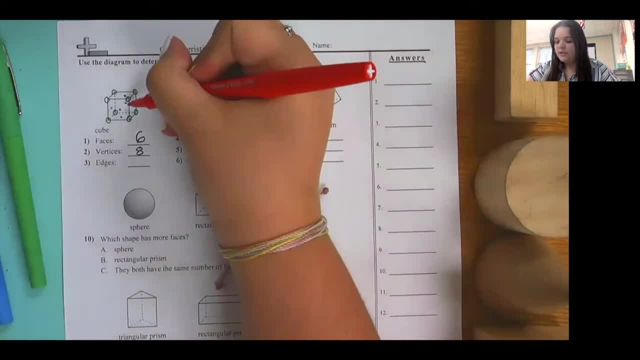 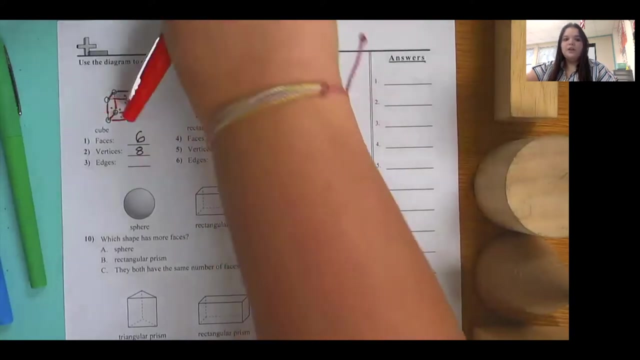 let's just call them the long ones. So the long ones. let's count them together: One, two, three, four, five, six, seven, eight, nine, 10,, 11, 12.. Good job guys. 12 edges. Hope you guys are. 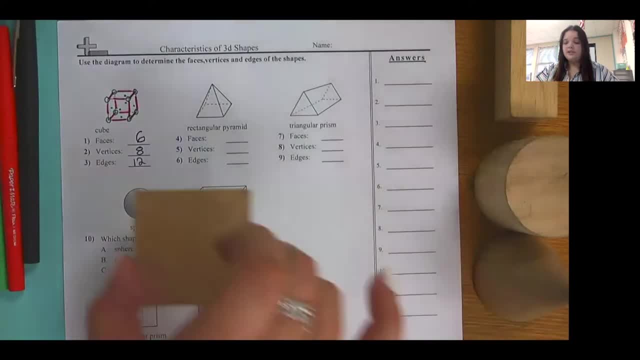 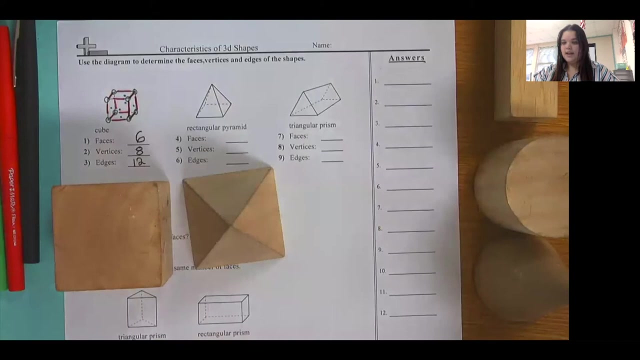 following along. Now we can also do this using our figure, which you guys should have on your desks. So you should have a cube, a rectangular pyramid and a triangle prism right here, just like that. You guys should all have one. Now we're going to do the rectangular pyramid using the rectangular pyramid. Let's 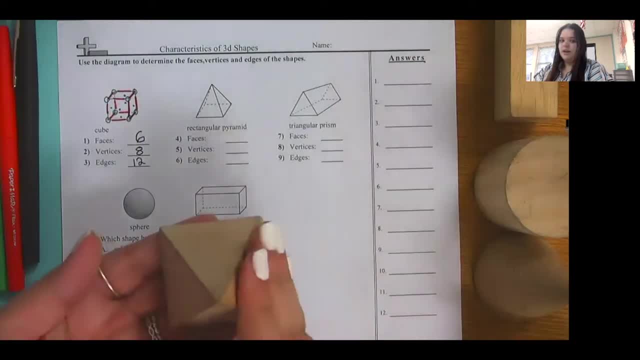 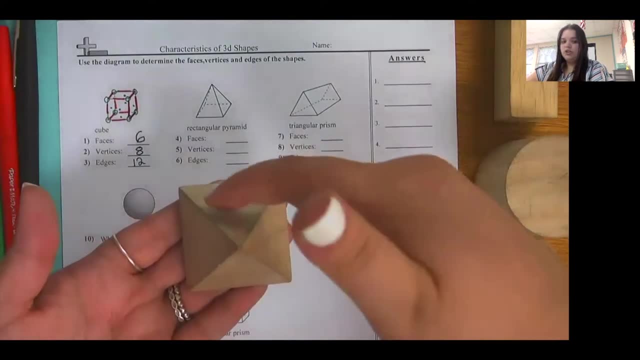 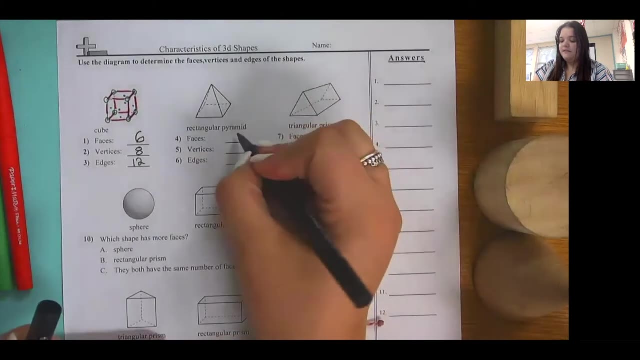 take this out. So we're going to go all right, faces- How many faces do we have? So let's count all together: One, two, three, four and five. So we have five faces. Now, if you wanted to do this in the paper, 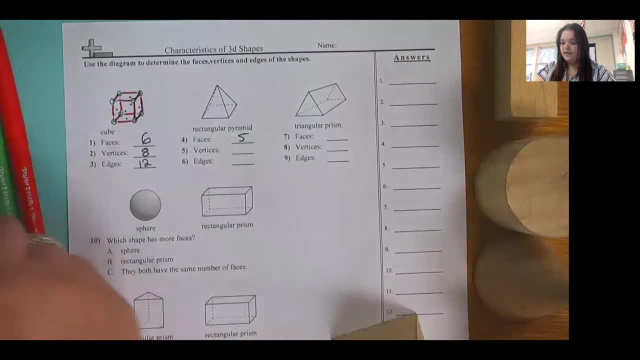 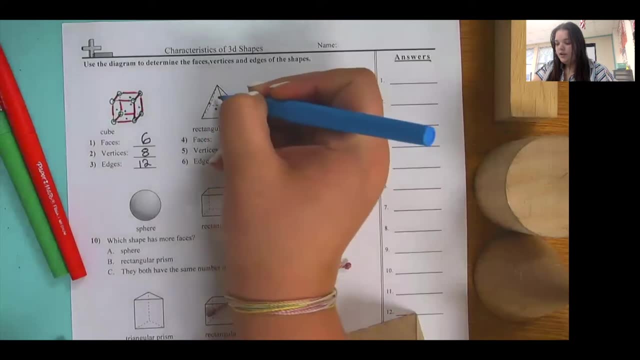 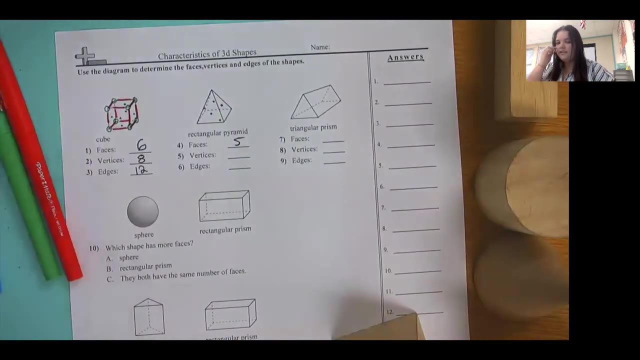 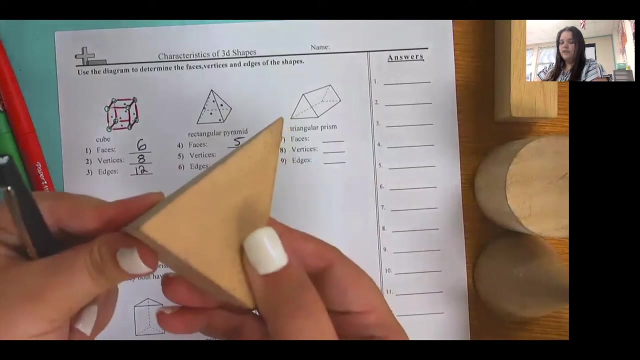 you could do the faces. We could do one, two, three, four and then the bottom one, five. So that's how you get five faces. The faces should be a little bit easier for you guys to tell on the actual solid figure than on the paper. Now the vertices and the edges should be easy. 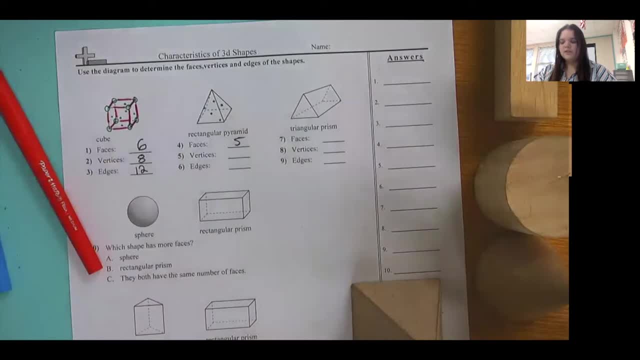 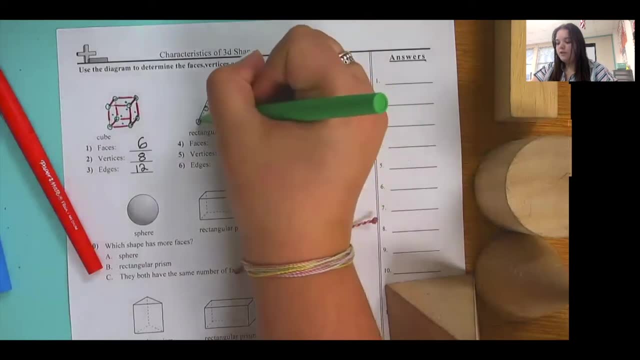 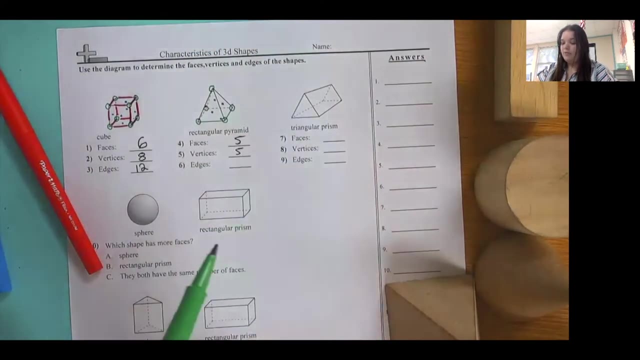 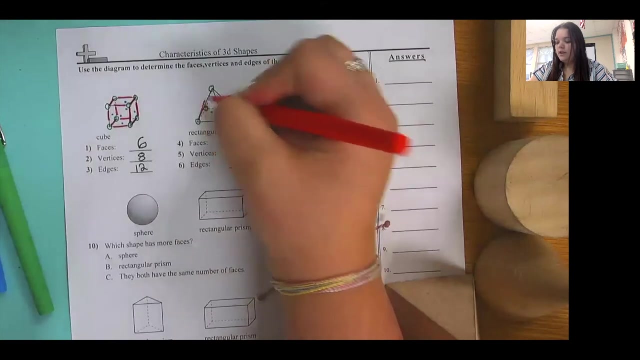 So how many vertices do we have? Which ones were the vertices? The corners? So we're going to go one, two, three, four and five, Five vertices. Now, how many edges do we got? That's easy, We already did it, Let's do it one more time. So we have one, two, three, four. 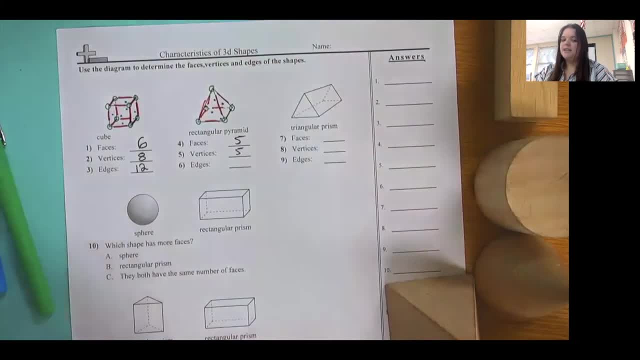 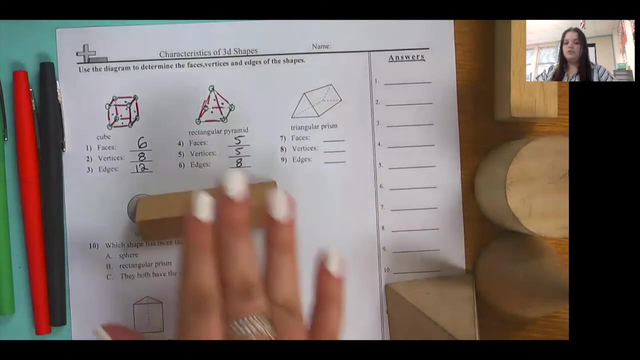 five, six, seven, eight edges. Good job. Now we're going to do one more. We're going to do this one right. So we have. let's do it with this first. Let's do it with the solid first. 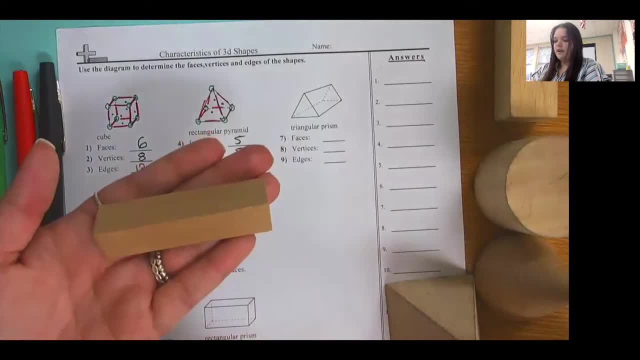 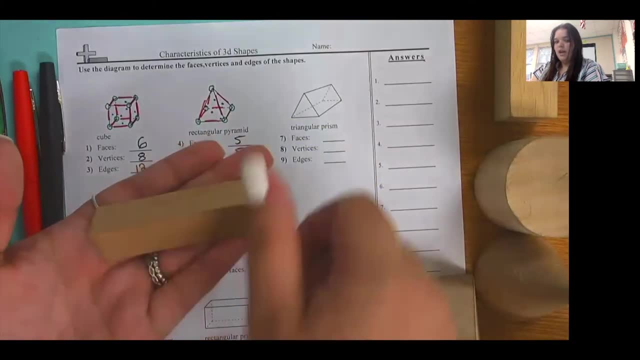 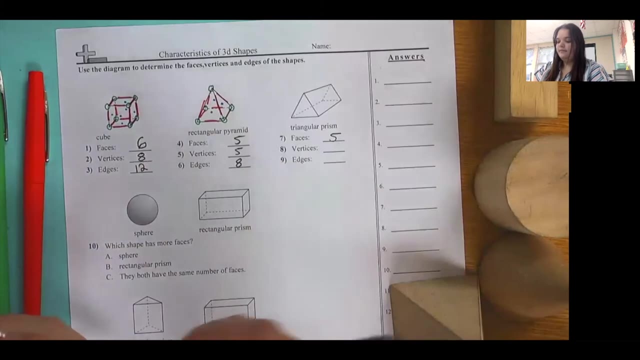 Now let's count how many faces we got. So we got one, two, three, four and if you turn it, five, So we got five faces. How many vertices do we got? So we got. let's count What were the vertices: The corners. 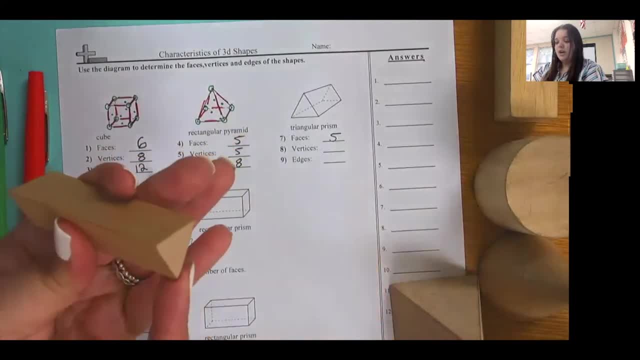 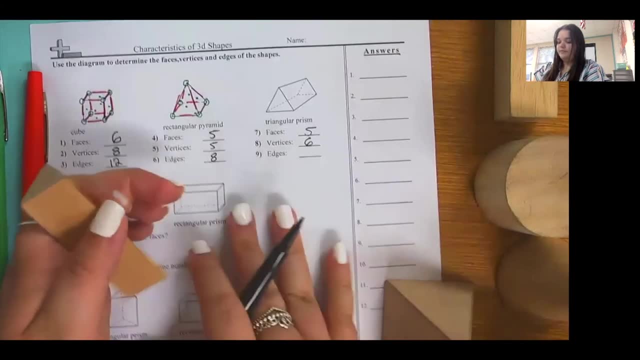 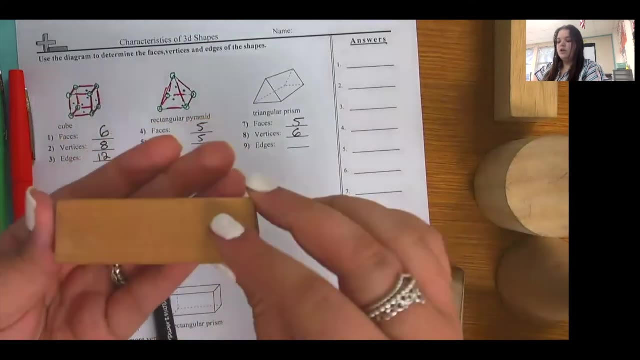 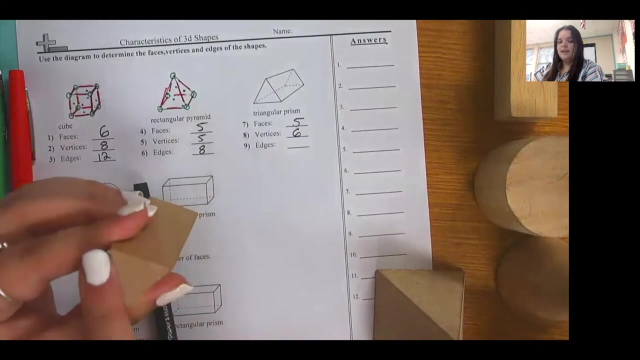 We got one, two, three, four, five and six. We got six vertices. Now let's count the edges Edges. We got one, two, three, four, five, six, seven, eight, nine. Good job, We got nine edges. 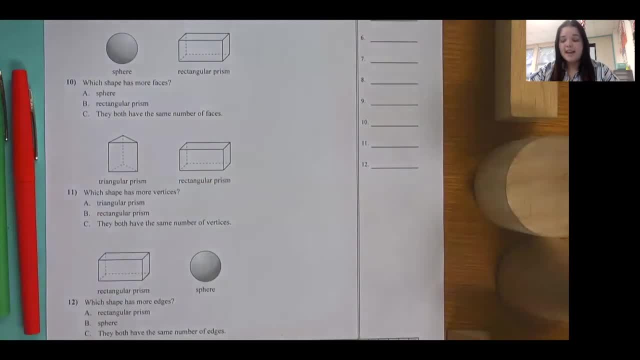 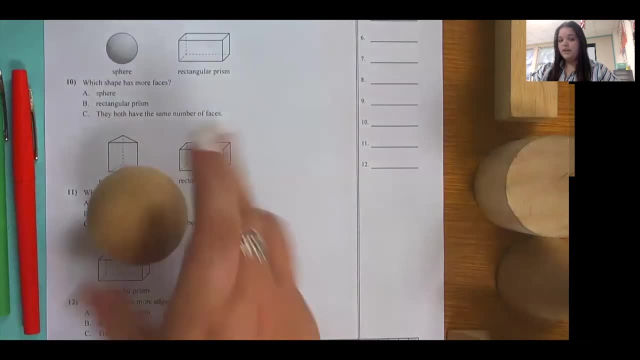 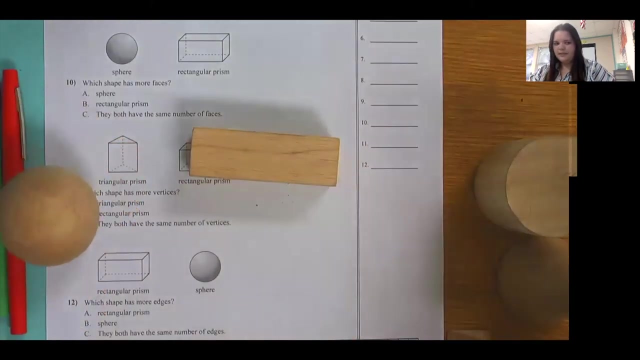 Right Now we're going to do this. last three. Let's read what the 10 says. It says which shape has more faces? So you have a sphere- You should have it on your desk- And we have a rectangular prism. So which one has more faces? 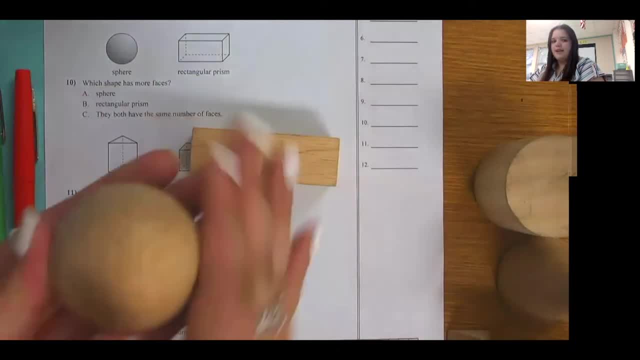 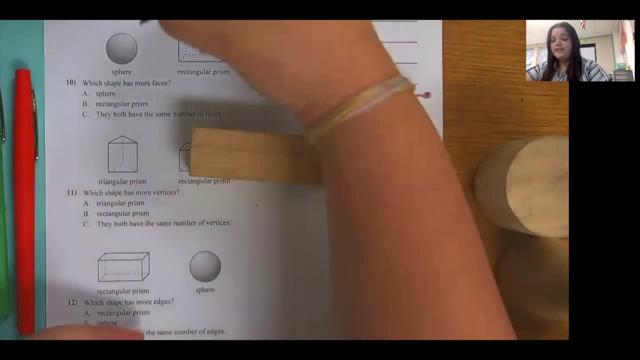 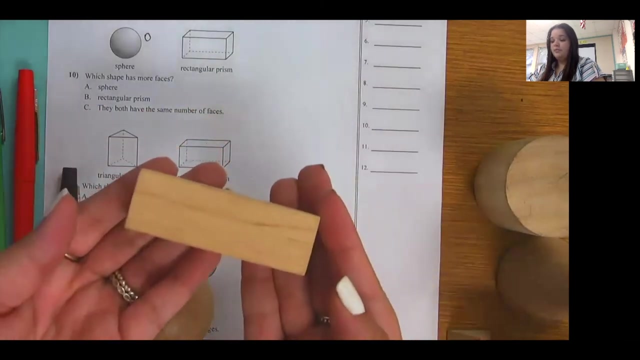 So we know that this one doesn't have faces. This one only has a base, which is the flat surface, but it doesn't have a face. So we know that a sphere has zero faces. Let's put a zero in that corner. Now, how many faces does the rectangular prism have? 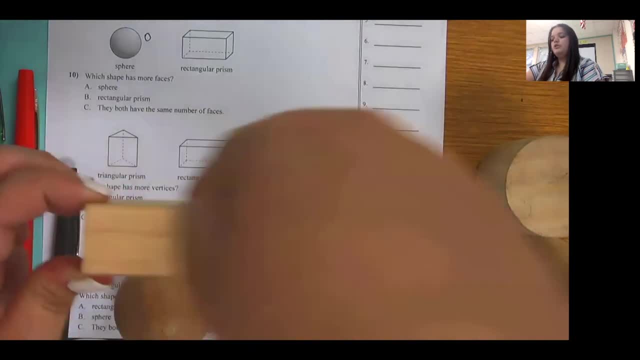 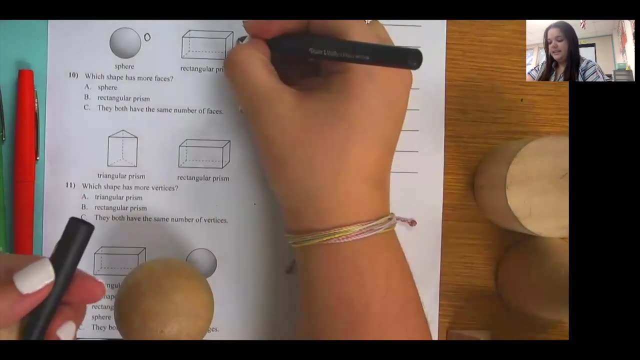 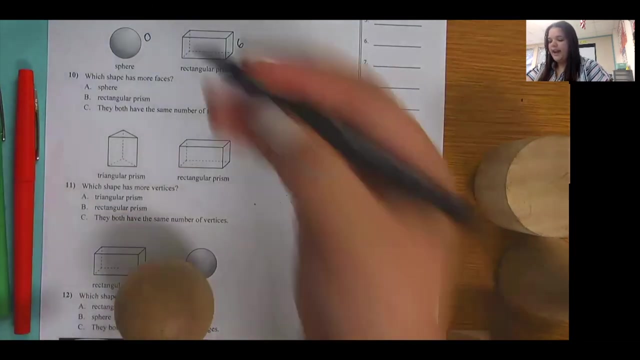 Okay, So we know we can count that. So we go: one, two, three, four, five and six. So this one has how many faces? Six faces. So that means which shape has more faces? The rectangular prism. Good job, All right. So this right here is your.